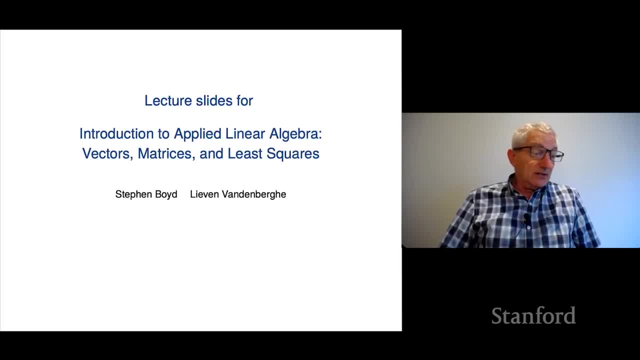 about that. You do not have to be like an expert programmer, Uh. you don't have to take in maybe a whole full course on computer science. Um, but you do have to know a little bit. Um, and I'll- I'll- I'll say more about that, uh, later. 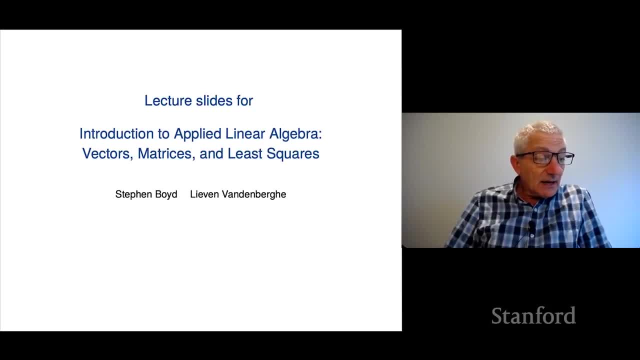 Um, okay, So let me say, uh, about how I- I think, uh, you can use these resources. So one- one resource is the book. I should mention that the book is actually just available online. You just go to Google or your favorite search engine. 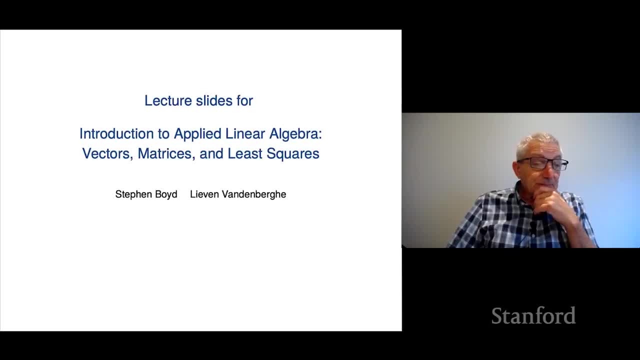 you'll find it pretty quick, uh, the PDF, uh file of the book. Um, and that's uh that's courtesy of Cambridge University Press, who were open-minded enough to uh allow us to post the book online. 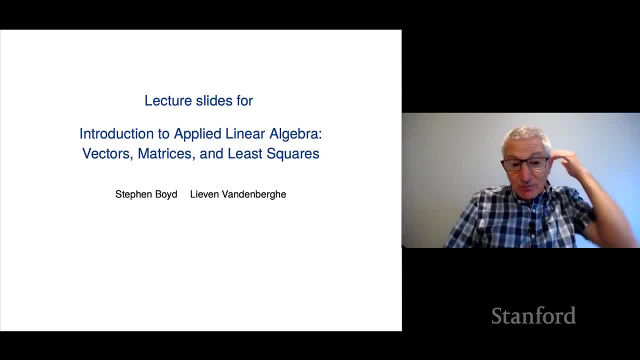 which I think is wonderful. Um, in fact, I even use the book uh online as well. I have, obviously, hard copy, but I use it online too, because there's links and you can jump from one place to another in search. 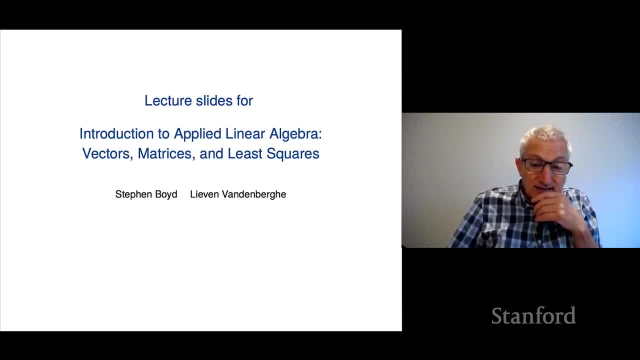 Uh, so, just everyone should be aware, the book is online, Um, uh, also online, you'll find these slides, the slides that I'm gonna cover, Um, and eventually you're gonna find, uh, these lectures as- as well. 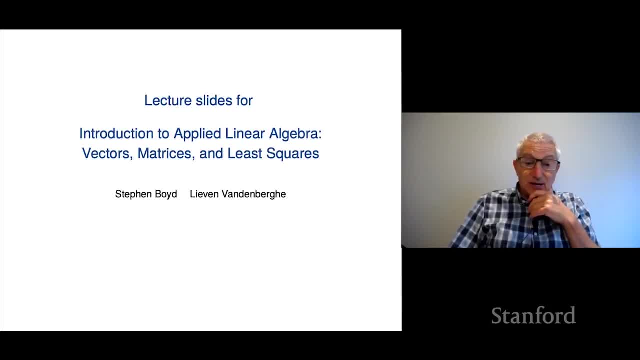 uh are gonna be uh online, uh, so posted for anybody in the world uh to- to watch Um. okay, So let me say a little bit about these the- the- the different um resources. 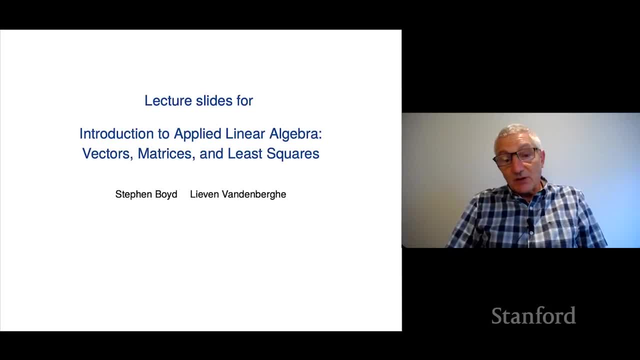 and- and how. I think, um, what the best, you know what- what might be a good way for you to learn? So, first of all, the book is- is complete, So you can read the book, and you can read it like a conventional book. 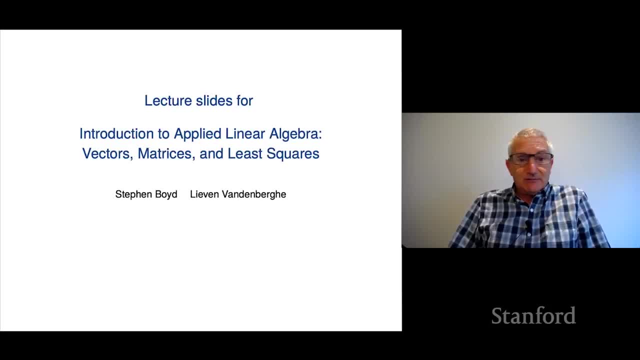 In other words, you could, uh, you know, read a chapter and you know whatever I mean. it's- I- it's readable, I think. So you can just read it, Um, and in fact that's a- that's a good thing to do. 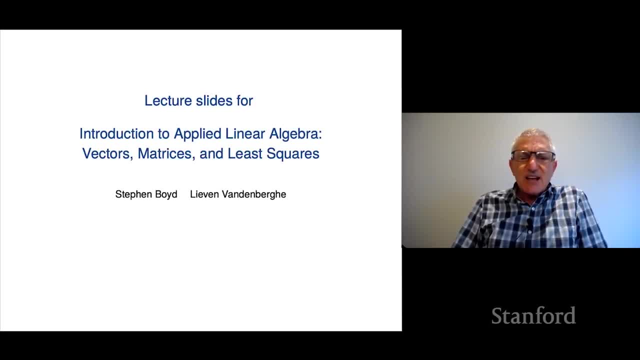 Uh, you know so. uh, it may not be a take it to the beach book, but it is kind- you know, maybe kind of a- of a windy and cold afternoon. uh, reading book could- could be perfectly good for that. 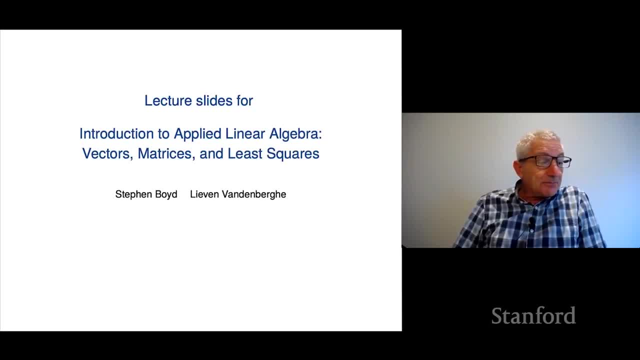 Just- just the book, Just read it. turn the pages, page to page Um, and it- it's of course the most detailed. It's got pretty much everything- uh in- is in there. So you know that- that's where- that's where you'd want-. 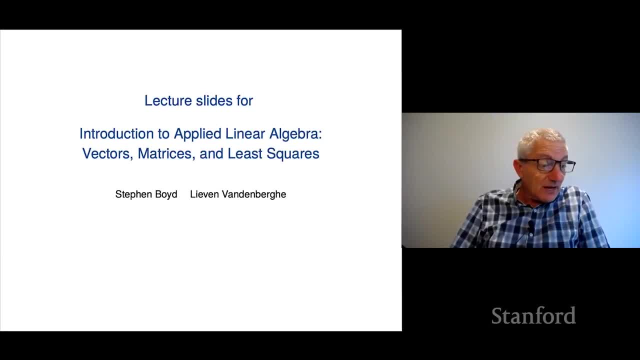 and we're very careful in our language in the book, relatively careful. Um, the slides are- well, of course, they are a condensation of the book, so they are more terse. Um, in some ways there's- there's something like the essence, uh, of the book. 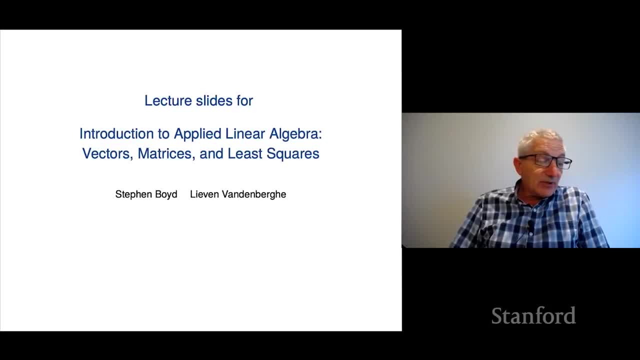 Now, not everything is there, so we don't carefully define every- every notation and things like that in the slides. Um, but the idea is it's supposed to be at a- maybe a 5,000 foot level. uh, what- what the course looks like. 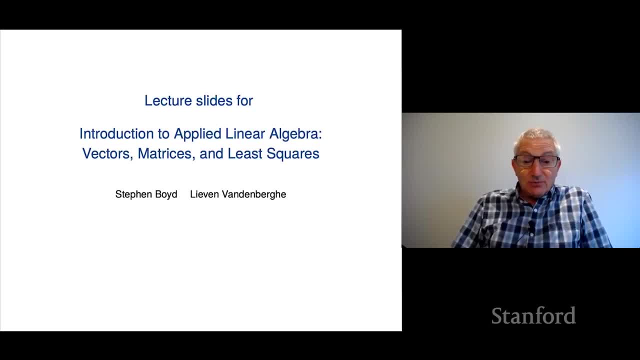 Um, and finally, there are these lectures. right, And you might ask you know, why would I listen to someone read the lectures? I can read perfectly well myself, That's true, And so the lectures are even, uh, more informal than the slides. 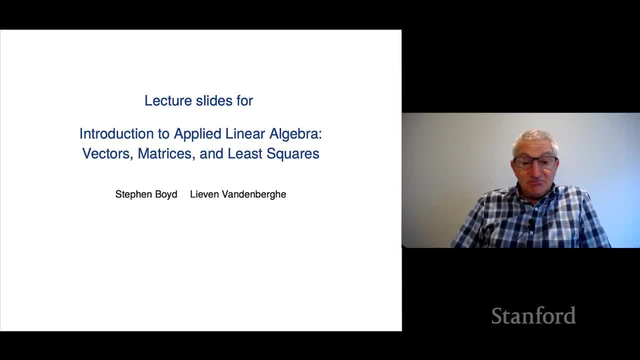 Uh, it's me, and what you get in the lectures is: uh, gossip, uh, st-. I might tell stories about various aspects, something like that: Um, of course it's not- it's not complete. uh, you know the- the- the lectures, uh. 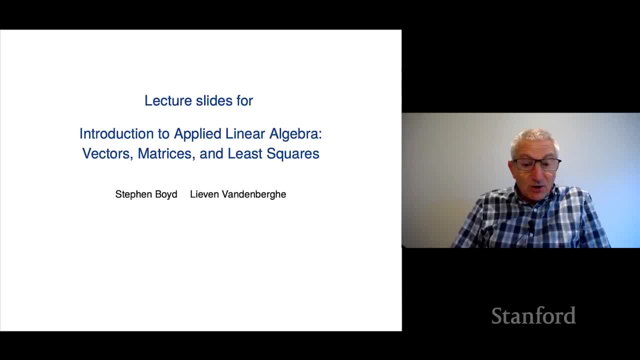 and you can't hold me to uh, you know, uh, everything won't be perfect and I- I may not defen- I- I might not define everything and all that sort of stuff. Um, so that- that's sort of- so how these three resources work for you. 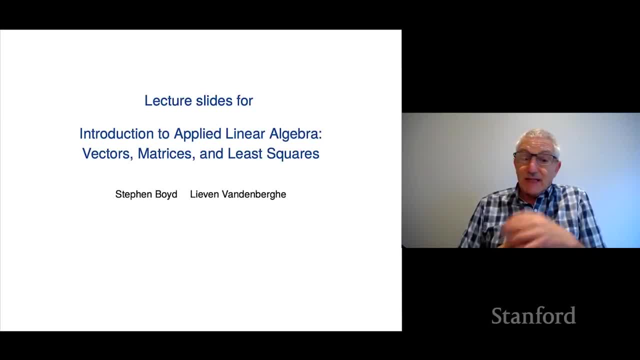 um, I think that that's very personal, depends on the person. Some people like to read like a chapter at a time, then look at the slides. uh, maybe watch the lecture, maybe the other way around: watch the lecture first, totally up to you. 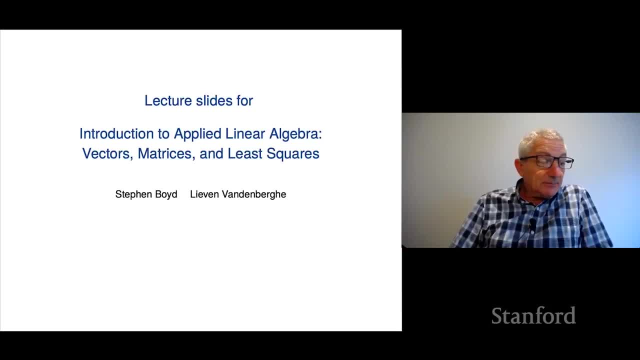 Actually, uh, honestly, I think all of these methods, uh, these work. Um, this brings me to something very, very important, um, and that's this: that the material that we're going to uh be covering uh in- that we cover in the book. 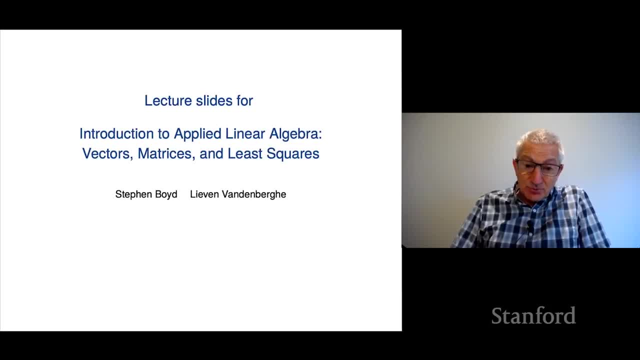 um, is super interesting and it is super useful And, in fact, one of the- one of the most important parts about it is that it's all actionable. It's not just theory. I mean, it is theory. There's beautiful theory. uh, that we're gonna- that we're gonna look at. 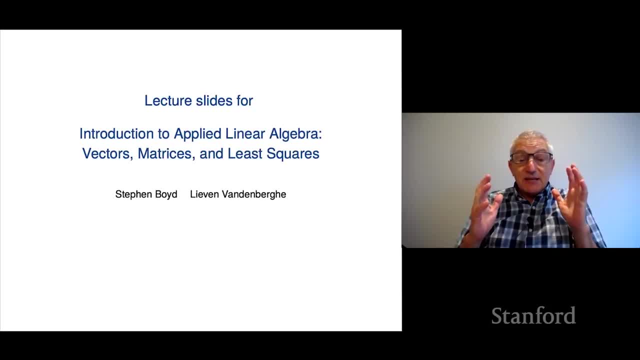 But the- but the really cool part about it is: you can do it. it is actually empowering and it enables you to do all sorts of crazy stuff. Um, you can fit models, uh, like in machine learning. We'll see other types of things you can do. 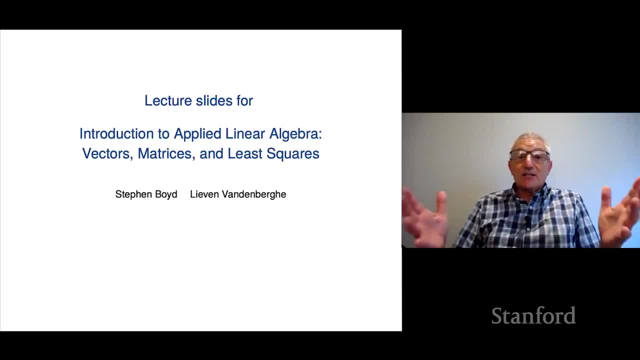 We can do uh signal processing, where you can extract a signal from a noisy signal. You can uh, you can do all sorts of stuff. You can uh model-. you can model epidemics, for example, using some of the material that we're gonna look at. 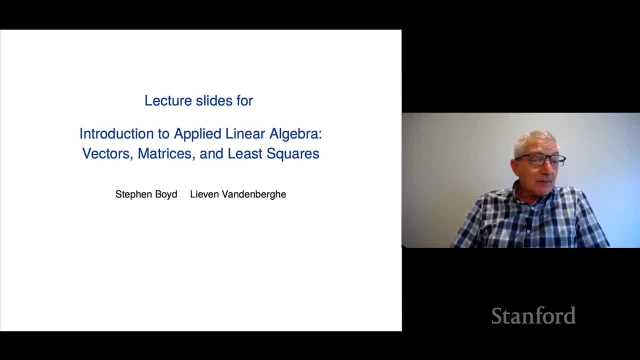 uh, in- in- in the course, So you can do a whole lot of stuff. Um, and it's very important in- in my opinion, it's very important that you follow along the book and the course. uh, doing numerical exercises in some computer. 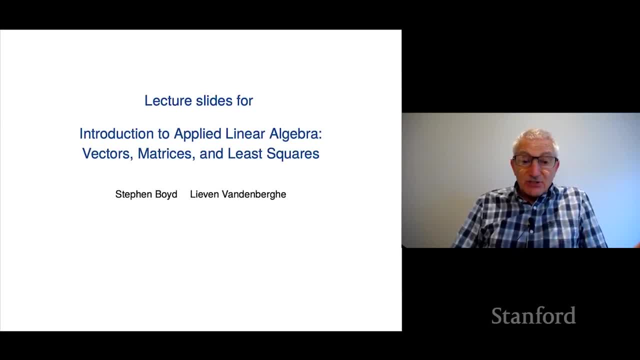 like language, Um, and even if that's not your interest, uh, even if you're interested, just to learn the theory, let's say: um, this helps enormously because it- it- it will actually jus- it'll help you go over in a different way and understand in a different way that topics. 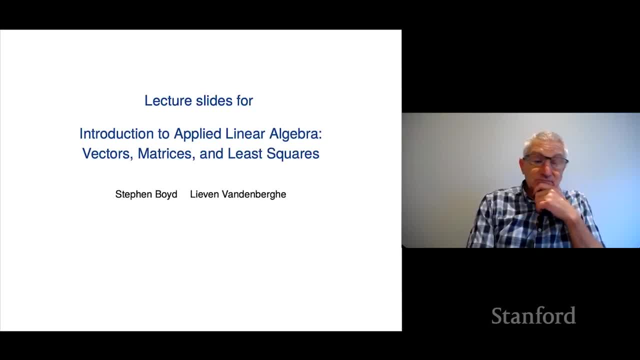 we're talking about. So you know, if I show you an identity, uh in you know an equation that is supposed to always hold. don't believe me, Just go to your favorite computer program. type in, you know. 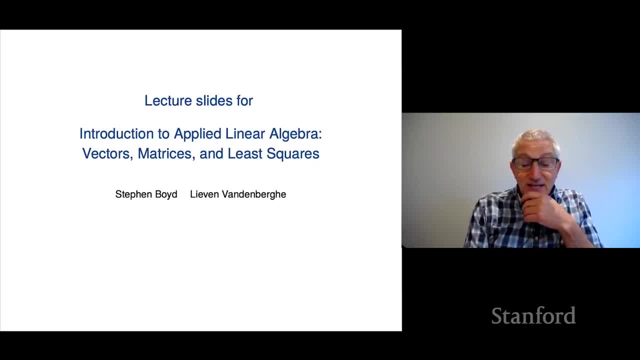 type in uh, something on the- type in the left-hand side to- type in something on the- type something type in the right hand, right hand side, and they should be, they should agree or be very, very close numerically, right. so this is, it's really uh great. uh to that i would strongly recommend, even though 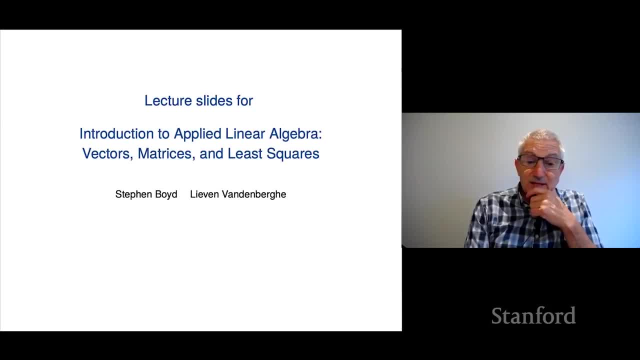 it's not necessary. you can read the book from cover to cover and we actually mention in the book no specific computer language. um, and i think you could actually- i mean it'd be, it'd be fine if that make that. that would be treating it as a conventional math book, but i think you'd really. 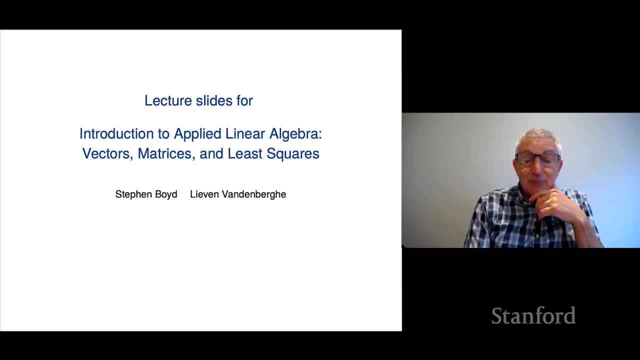 be wasting um a an important uh opportunity here, uh, which is that the material of this course is actually actionable. you can actually do it. or i like to say this: uh, linear algebra should not be a spectator sport. so jump in there, get your hands dirty, fire up one of these tools and uh follow. 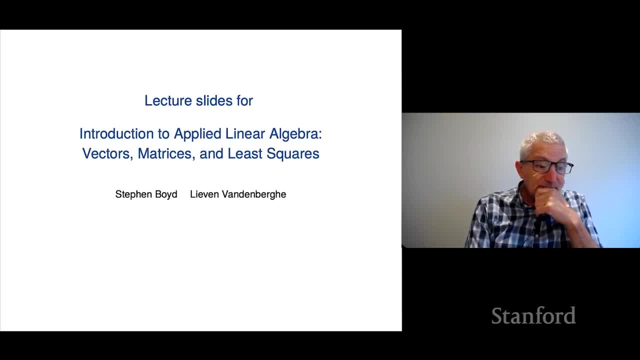 along that way. i think that that'll help a lot. um, i should add, that's going to be super important when you you know if you end up doing a summer internship or something like that where you use these things. it's one thing that's going to be super important when you you know if you end up doing a summer internship, or. 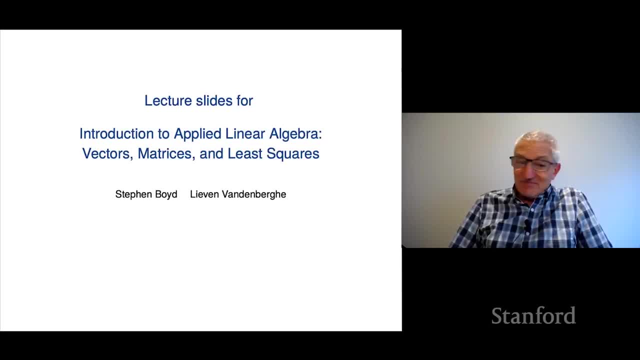 know the material in this book. it's quite another to be able to sit down and actually do something with it, which is very, very cool, um. so let me say a little bit about languages. so in at the stanford course, uh, we, we happen to use julia. that's a, that's a relatively new uh language. 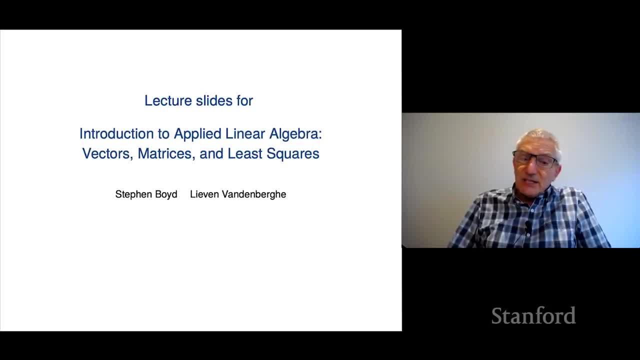 and you know the reason is it. it works super well, but it's also, um, it's the one that maybe has the notation that is kind of closest, uh to ours. um, another one, uh, that is an option, is matlab. uh, now, that's proprietary, meaning that you'd have to, you'd have to pay. 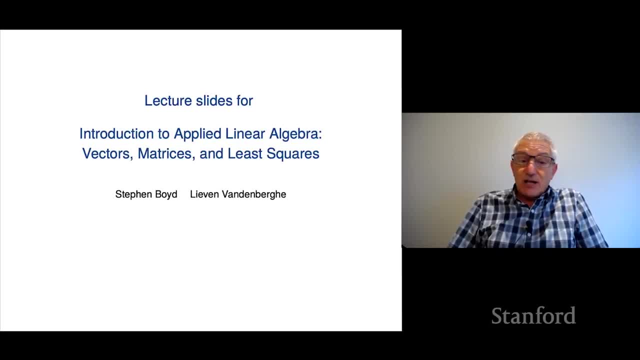 for it, um, but it is a perfectly good option to follow along with the ideas, uh in in this course. um. and the last another option, um is python. python's an interesting option, and i do know that some people are teaching this course, uh, teaching a course based on the book, and they're 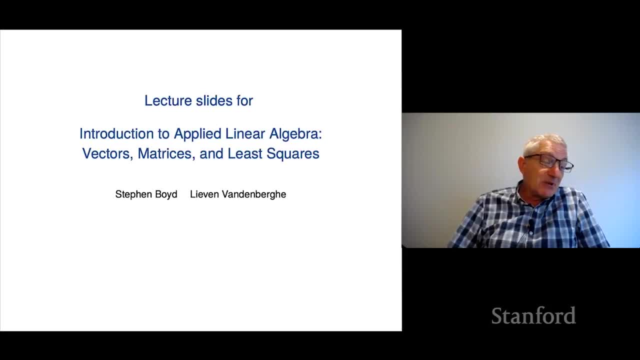 using python, and it's actually a perfectly good choice, and the reason is that most people these days are using python to do the kinds of stuff that you're going to learn about in the future in this course, so in some sense, it makes sense for you to uh to start start off um with the uh. 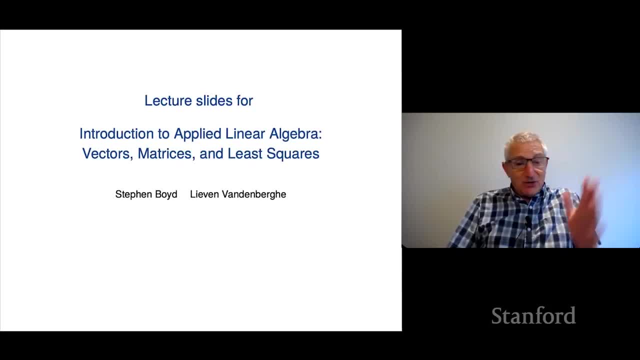 with the language that you'd actually use in your internship or your job or your startup. um, so that would be the argument behind python. uh, my only reason for not selecting python in my own course, um, is that the syntax is a little bit, uh, clunky and it deviates a little bit from the 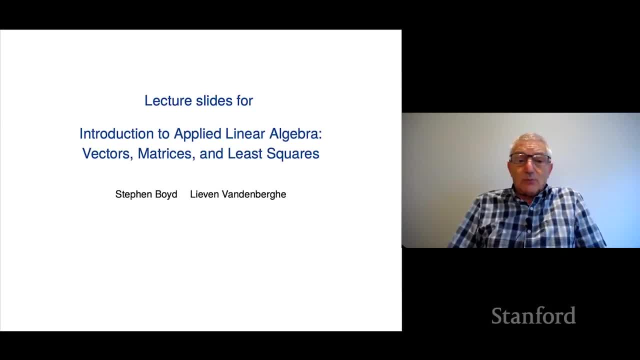 from the mathematical syntax. uh, not in a terribly horrible way, but it just seemed to me that julia, uh the julia language syntax fit the ideas just a little bit better. but anyway, overall, though, i would strongly urge you to uh to follow along this course. uh with us with doing some numerical 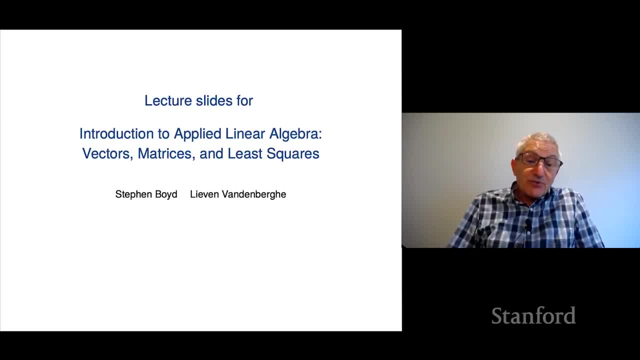 examples. now the book itself does not refer uh, or refers only a few times to uh computation. it does describe a little bit about computation but we don't mention any specific computer language in the book. um, there will be a few exercises. there are a few exercises in the book.